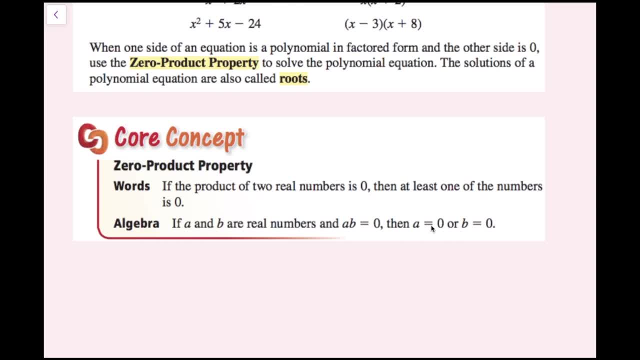 then a equals b, b equals zero or b equals zero. So at least one of these has to be zero. So we can either do zero times zero, zero times b or a times zero. Any of that would make that equation true. 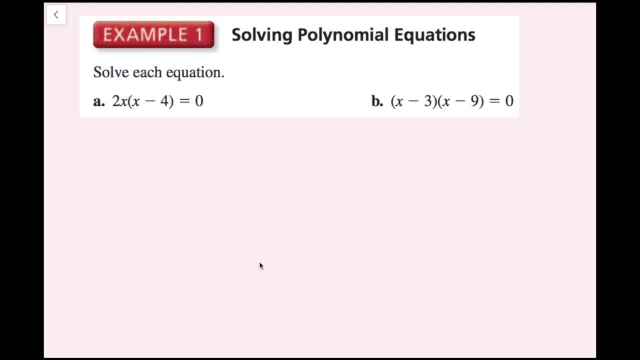 So in this example we're going to be solving the equations. Well, for part a, I have 2x times the quantity x minus 4 equals zero. Well, this is an example where I can use my zero product property. okay. 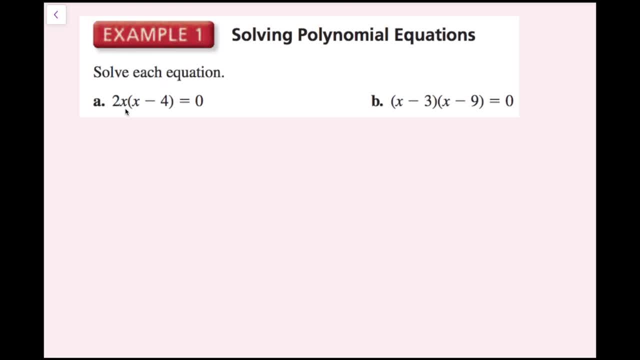 Well, I have something times something else and that's going to equal zero. So that means that at least one of these things has to be equal to zero. So I'm going to break this up Into: 2x is going to either equal zero, or x minus 4 is going to equal zero. 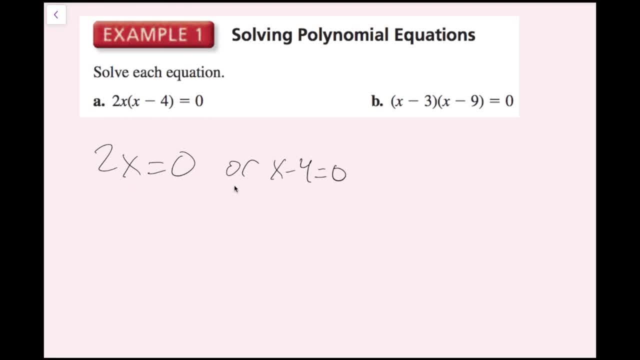 And then I just have to solve these equations to find my x values. So here I can either divide by 2 on both sides to get zero for x, or you can just think what number times 2 is equal to zero. That has to be zero, okay. 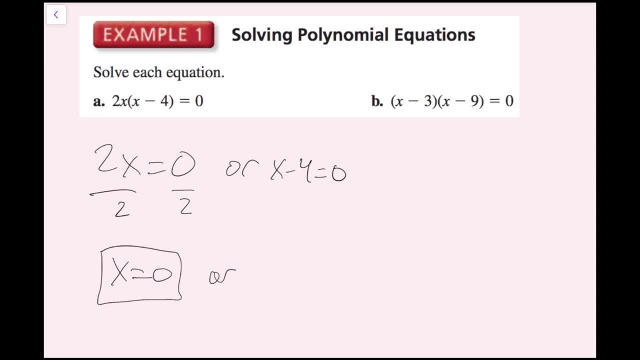 So x equals zero is one of my solutions. Or, and then here all I have to do is add 4 on both sides and I get x equals 4.. So I can write it like this. or I can write my values like this: 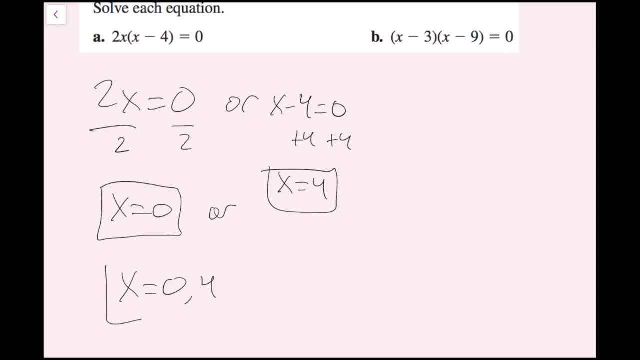 x equals zero 4.. Either this way or this way will work And, using our vocab term, one way we can say this is that zero and 4 are the roots of this equation. For part b, I'm going to do the same thing. 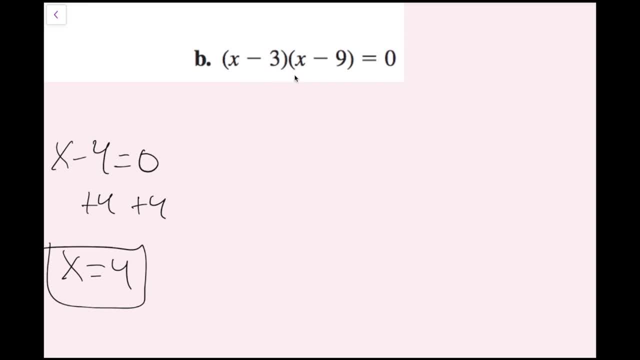 So I'm going to zoom in here. So I get x minus 3.. This quantity is being multiplied by the quantity x minus 9.. So this thing times this thing equals zero. At least one of these has to be zero, So I'm going to rewrite this as x minus 3 equals zero. 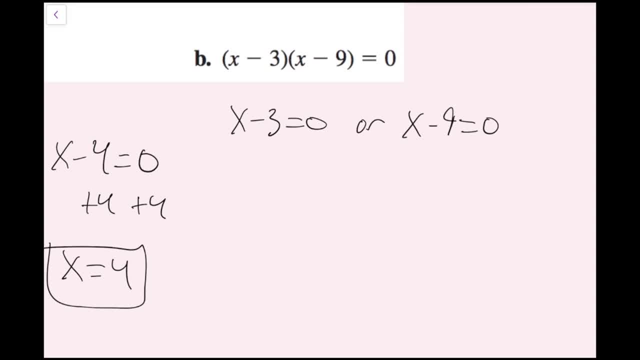 or x minus 9 equals zero. And then I'm just going to solve these equations. So if I add 3, I get x equals 3.. Or if I add 9,, I get x equals 9.. Once again, I can write it like this: 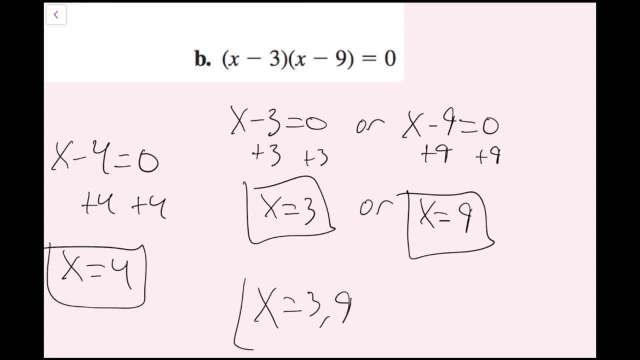 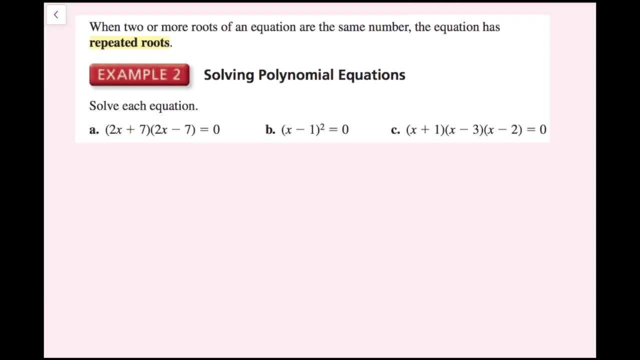 or I can write: x equals 3,, 9.. So my x values that make this equation true are 3 and 9, and now we're done. When two or more roots of an equation are the same number, the equation has repeated roots. 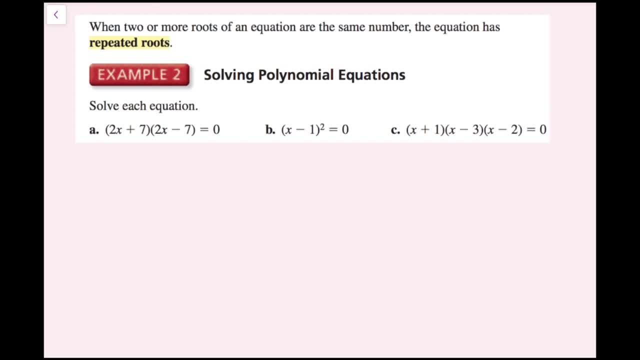 So, for example two, we're going to solve each equation and we're actually going to see an example that has repeated roots. So for part a, I have 2x plus 7 times the quantity. 2x minus 7 equals zero. 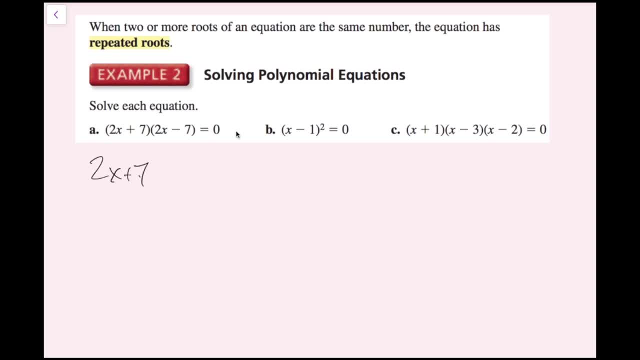 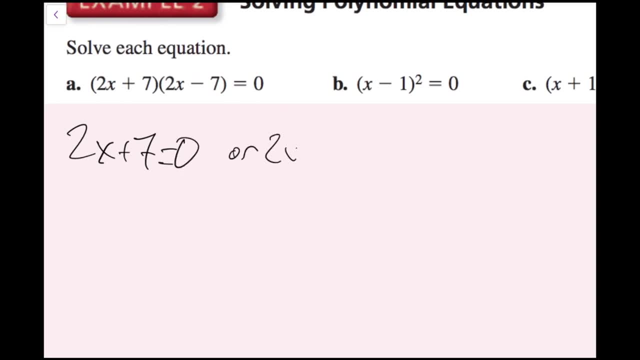 Well, I'm just going to set this: 2x plus 7 equals zero. I'm going to zoom in a little bit: write a better zero And then: or 2x minus 7 equals zero, Okay, well, I'm going to solve the equation on the left first. 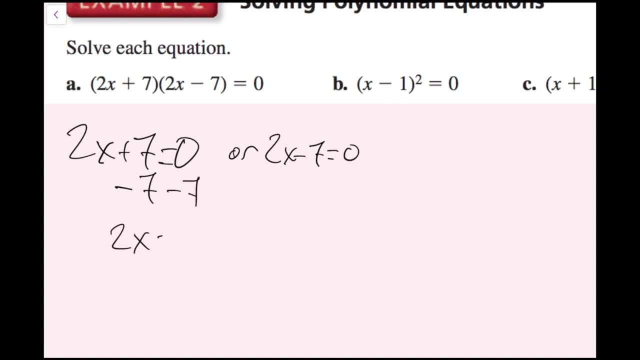 I'm going to subtract 7.. I get 2x equals negative 7, then divide 2.. I get x equals negative 7 over 2.. That's one of my values. If I solve this equation, I would add 7 on both sides. 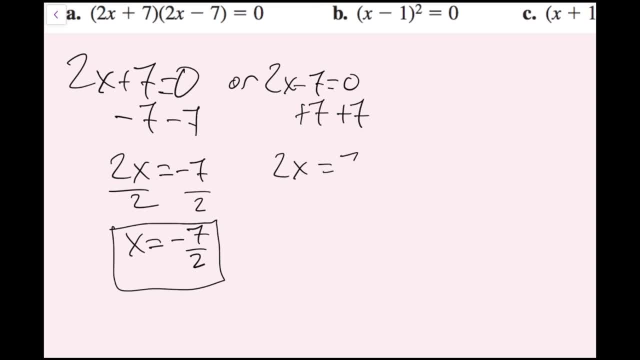 So I get 2x equals 7.. Then I divide by 2 right here, So I get divide: 2.. I'd get x equals 7.. Okay, you could write this as 3.5 or 3 and 1 half. 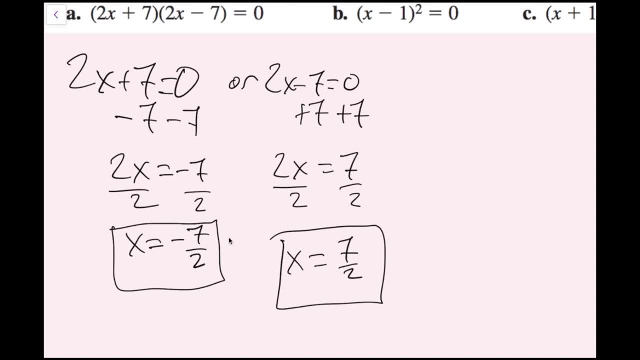 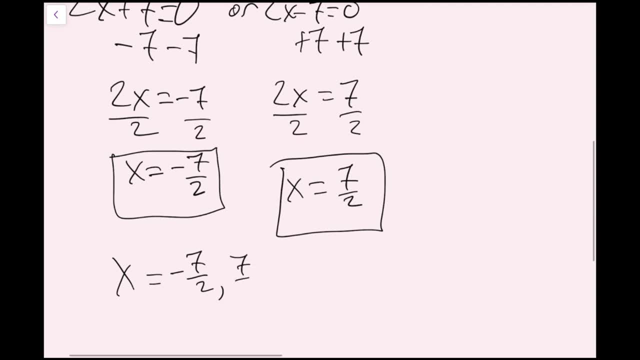 but I'm going to leave it as an improper fraction for now. Okay, so I could write it like this. I could also write it like: x equals negative 7 halves, comma 7 halves- I forgot my or up here- And I could also write it in a special way, because I have a number and it's opposite. 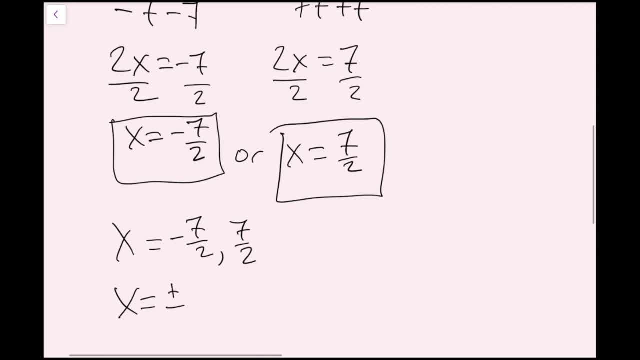 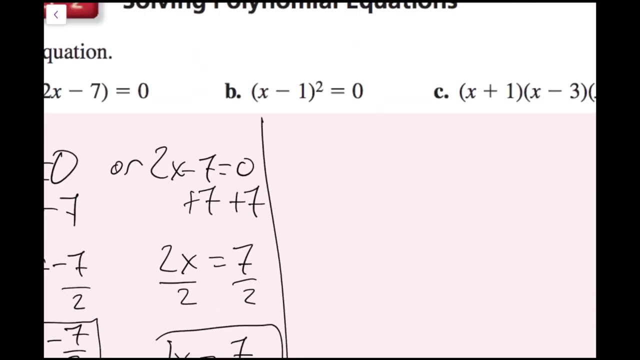 So I can actually write this as: x equals plus or minus 7 halves. Okay, and you'll see that later in this course. Anyway, we're done with part A. Now I'm going to move on to part B. So I have the equation: x minus 1, quantity squared equals 0.. 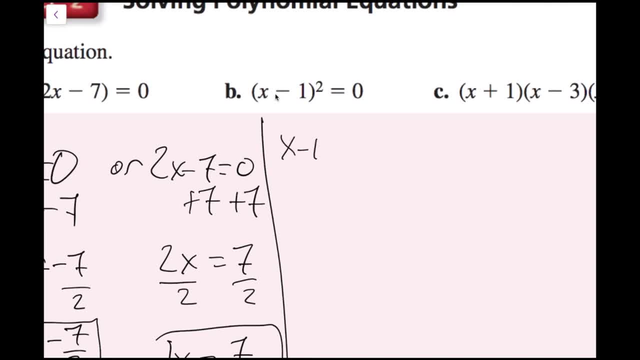 Well, I'm just going to write this out. This is x minus 1 times x minus 1 equals 0.. So if I was going to write my two equations to solve this using the zero product property, I'd write: x minus 1 equals 0.. 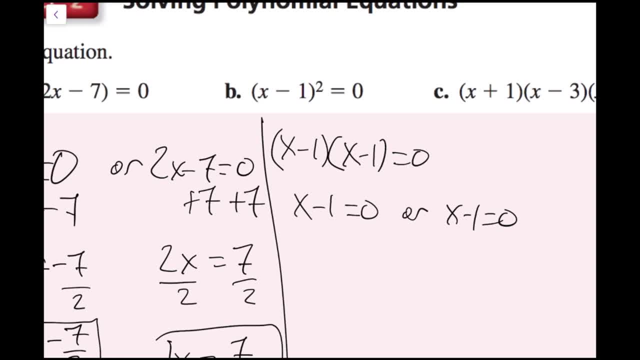 Or x minus 1 equals 0. And notice, they're the same equation, So I'm going to get the same answer. if I add 1 on both sides, I'm going to get x equals 1 or x equals 1 for both of them. 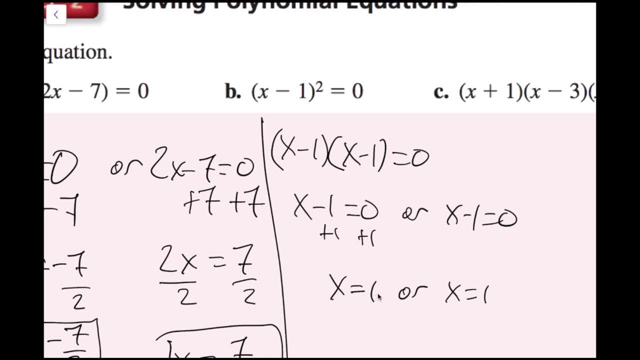 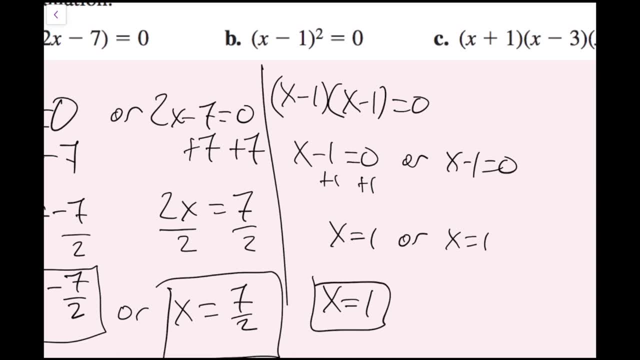 This is an example of repeated roots. Okay, so 1 would be a repeated root. So what you could say is: x equals 1.. And that's the only value that will make this equation true. So now we're done with part B. 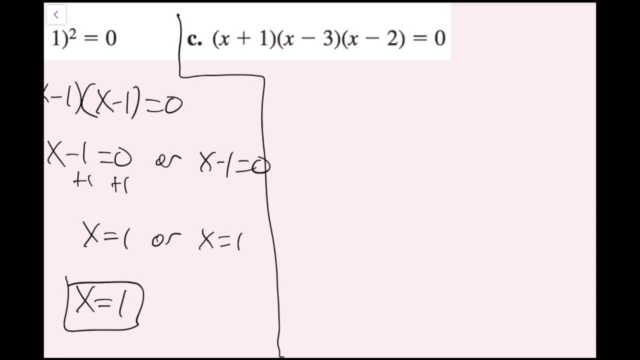 Part C. I'm just going to kind of give ourselves more space. I have x Plus 1, that quantity times x minus 3, times the quantity x minus 2.. Okay, well, there's more than two things being multiplied, but that's okay. 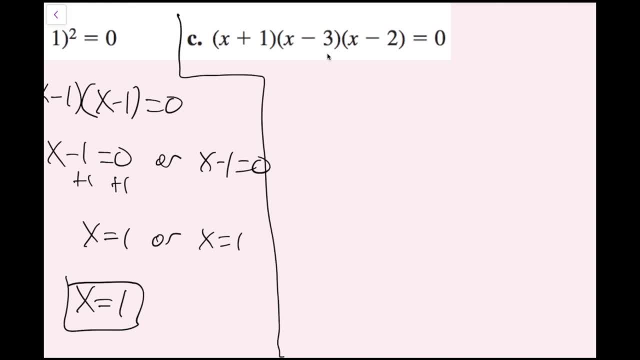 I'm just going to set all of them equal to 0.. So this x plus 1 factor, this x minus 3 factor and this x minus 2.. So I get x plus 1 equals 0, or x minus 3 equals 0, or x minus 2 equals 0. 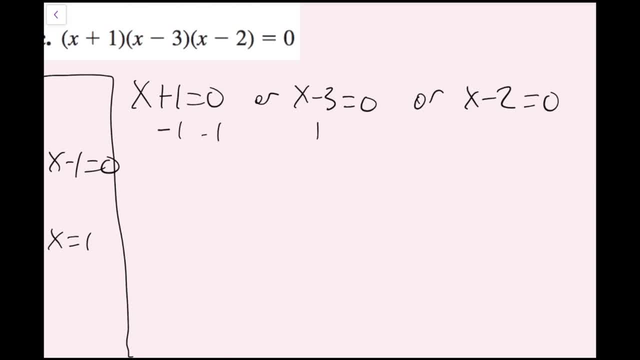 Okay, now I'm just going to solve all these equations: Minus 1,, add 3.. Add 2.. So I get x equals negative 1, or x equals 3, or x equals 2.. So these are my x values. 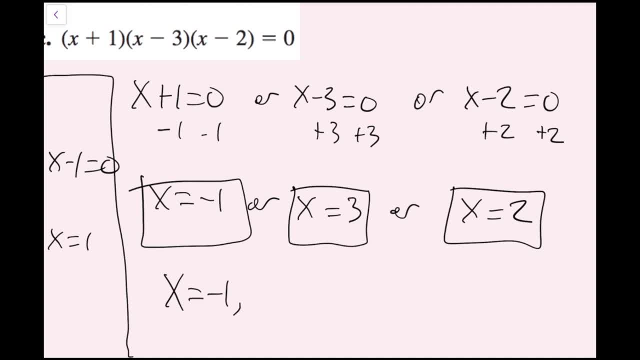 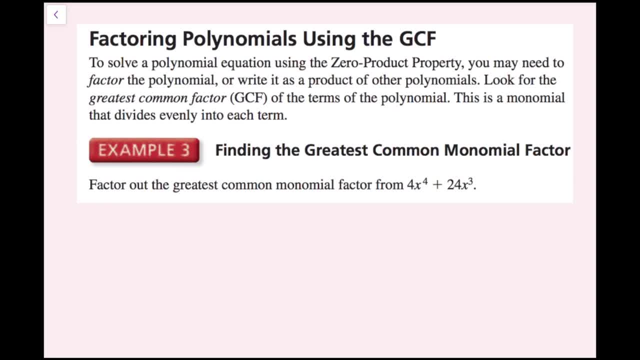 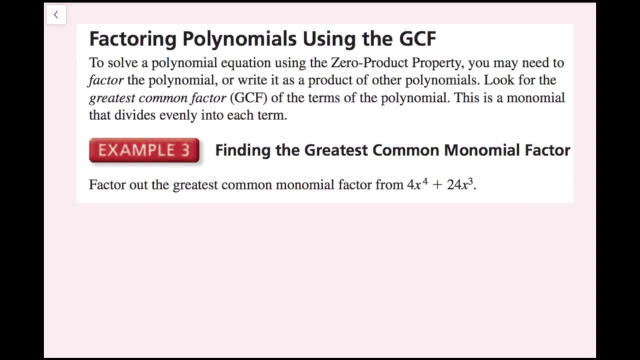 that divides evenly into each term. So, for example three, we're going to factor out the greatest common monomial factor from 4x to the fourth power plus 24x cubed. Okay, so I'm going to zoom in here. Well, in order to factor this out, I often like to use what I call the ladder method. 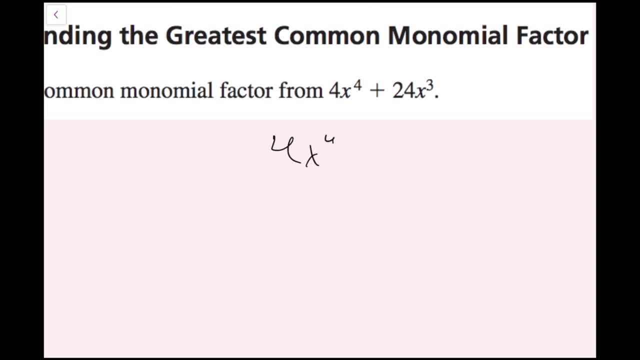 So I'm going to write 4x to the fourth and then plus 24x cubed, Okay. and then I want to see what I can factor out here. Now you can tell right away, if you want, what the greatest common factor is. 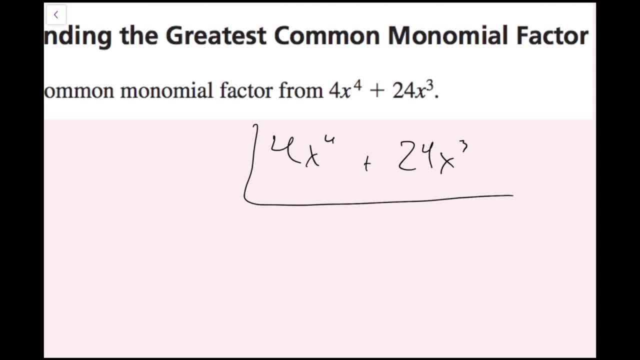 going to be, or you can factor things out at different steps. Okay, and I'll do both. So, right here I can get a 4 out of the 4 and the 24.. Okay, so if I do that, I get a 4, and then I get an x to the fourth is left over, plus 6x cubed. Okay, now I'm going to. 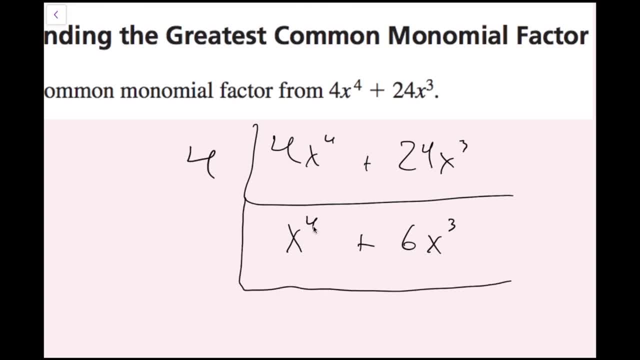 make another step in my ladder and I have x to the fourth power and 6x cubed. Well, this has 4x's being multiplied. This has 3x's that are being multiplied, So I know I can take out at. 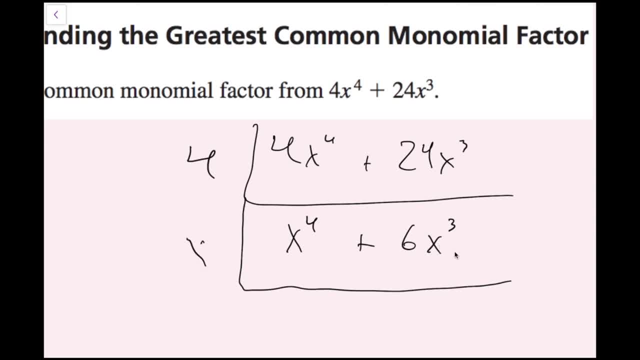 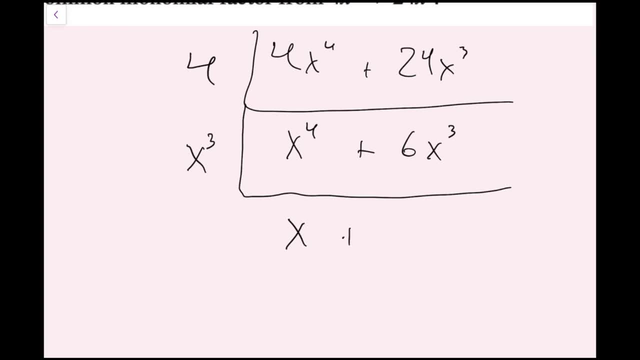 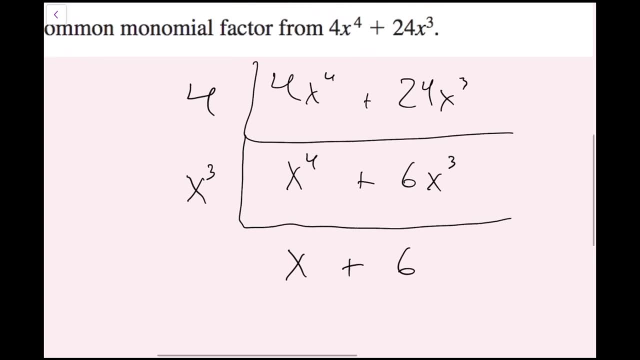 least 3x's that are being multiplied, So I get x cubed, and what I have left, just x here, because, and then plus well, I took the x cubed away, So now I just have 6.. Okay, so now what I have is x. 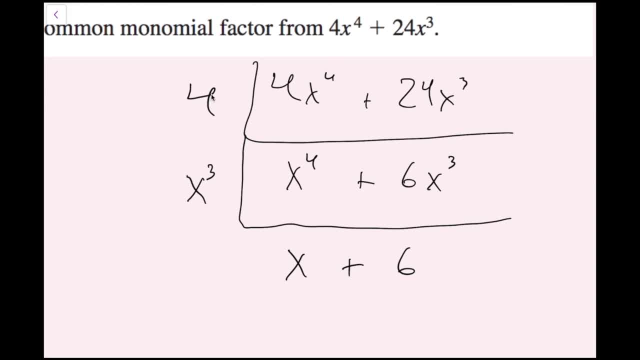 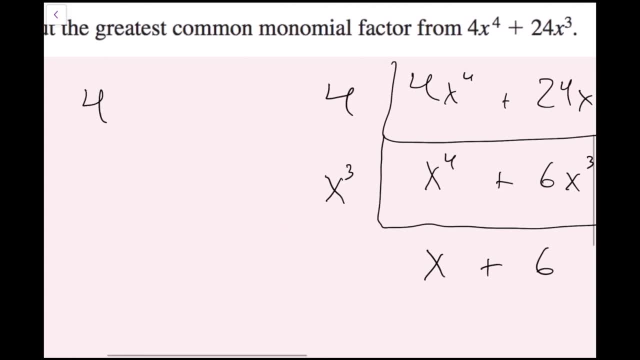 plus 6 is going to be left over. And then my greatest common factor is just: if I multiply this and this, well, I have a 4 and an x cubed. Okay, so this is going to turn into 4x cubed times the. 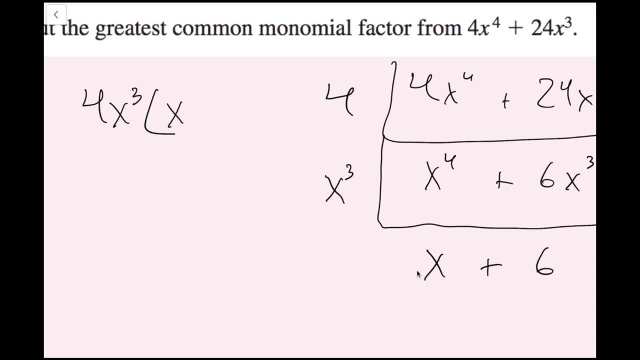 quantity. Well, x plus 6 is left over, So this is going to be x plus 6.. All right, so this ladder method right here isn't really going to be necessary, but this is kind of why it works And it could help you, especially as you're starting out. But if you don't want to, 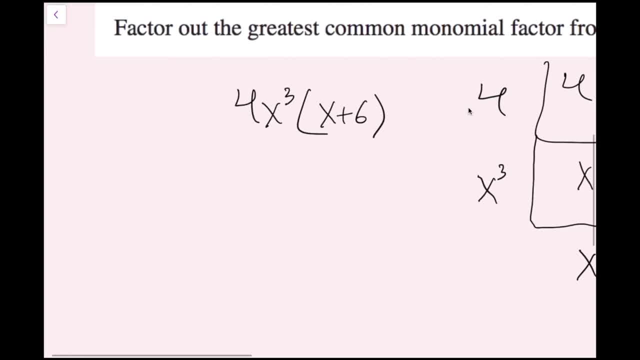 use that, that's totally fine. I'll show you that we can just kind of do that without making that ladder. So if I had 4x to the fourth plus 24x cubed, I can kind of just look at each term and 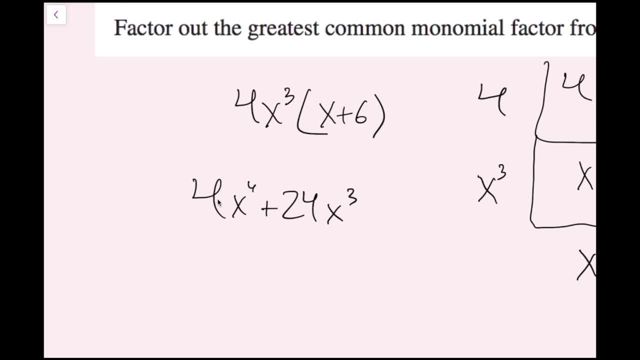 say: okay, what is the number greatest common factor And what's the variable greatest common factor? Well, the number greatest common factor is going to be 4.. And this has an x cubed. this lower exponent is: we can factor that out, And I'm going to get 4x cubed. And then I just want: 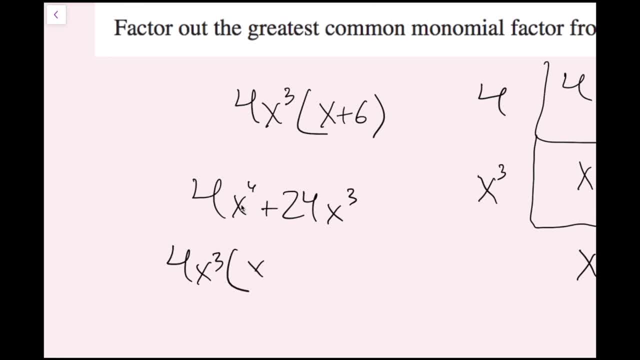 to see: okay, 4x cubed times, what is x to the fourth? That's going to be x plus 4x cubed times. what equals 24x cubed. Well, that's just going to be 6, because 6 times 4 is 24.. And then I just 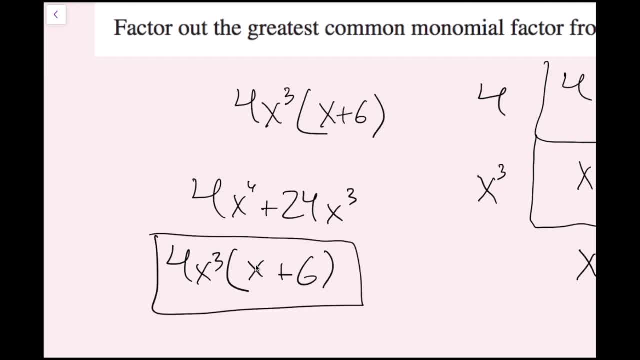 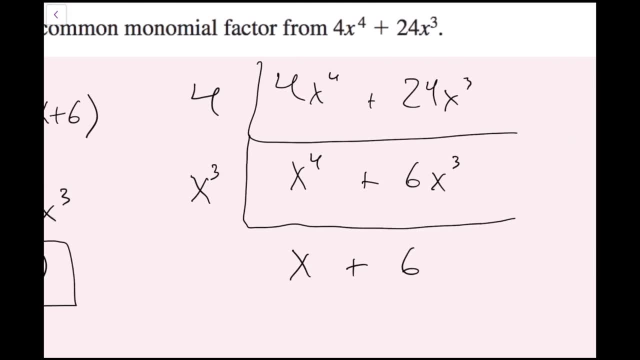 bring my x cubed term over. Okay, so this is our final answer. It doesn't matter which way you get it, The way I did it. second is probably quicker, but the ladder method can help you out, just as with problems like these. Anyway, now we're done with this one. For example 4, we're going to solve. 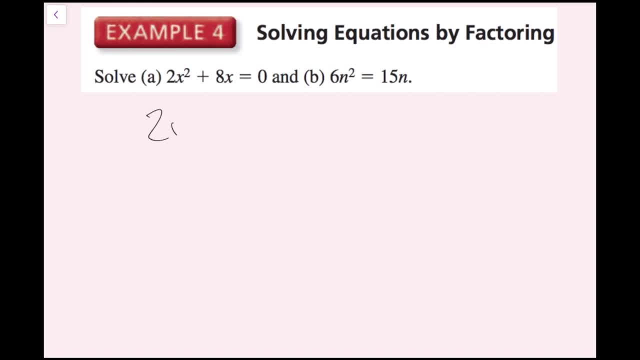 some equations by factoring. So for part a, I need to solve: 2x squared plus 8x equals 0.. All right, So what I want to do is factor out the GCF greatest common factor, And I can see right here. 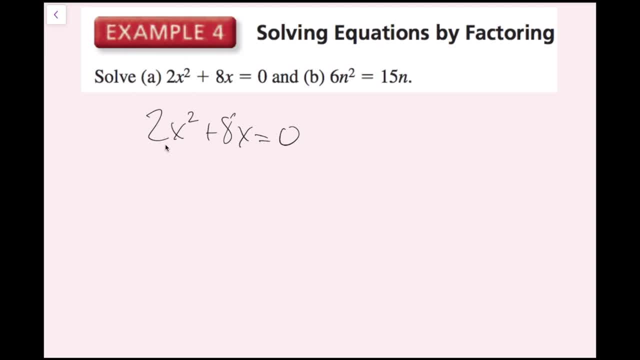 from these two terms I can factor out a 2, because they're both even, And then I can factor out an x, because this has an x and this has an x squared. So I can factor out an x, And then what's left? 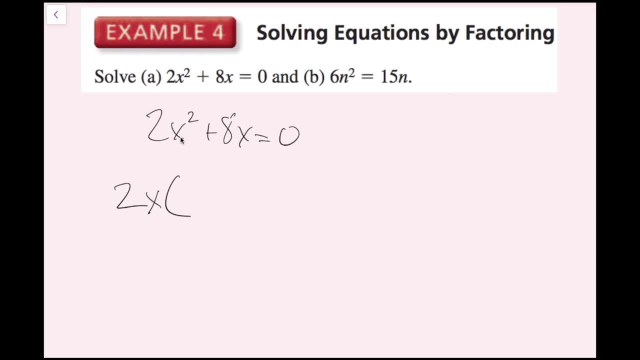 here I factor out, or you can think of it as dividing out- this 2x term. It's just going to be an x here, because 2x times x is 2x squared. And then, right here, I'm just going to have 4, because 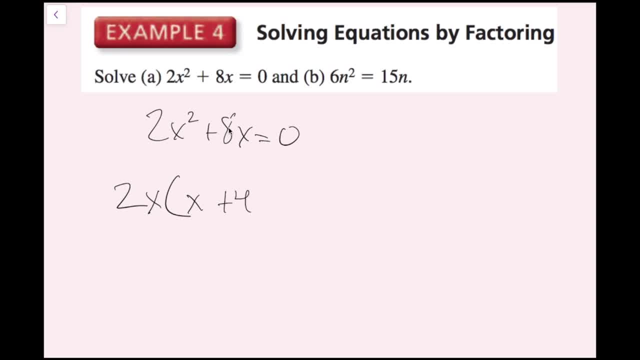 4 times 2x gives me 8x. So now I have a factored polynomial equation and I can solve this using the zero product property. So I have 2x and x plus 4.. So I'm going to set 2x equal to 0, and then x. 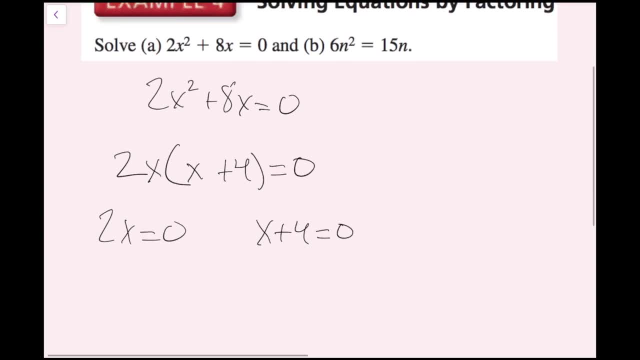 plus 4 equal to 0.. If I solve this well, if you remember, we did this before. So I'm going to set 2x equal to 0.. And then x plus 4 equal to 0.. If I solve this well, if you remember, we did this. 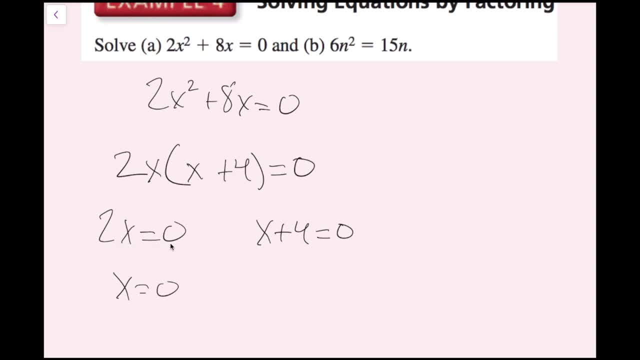 earlier, this is just going to be x equals 0. You could divide by 2 on both sides, or you could just tell: well, 2 times 0 is going to be 0. So that's my only x value for this one, Or I have x. 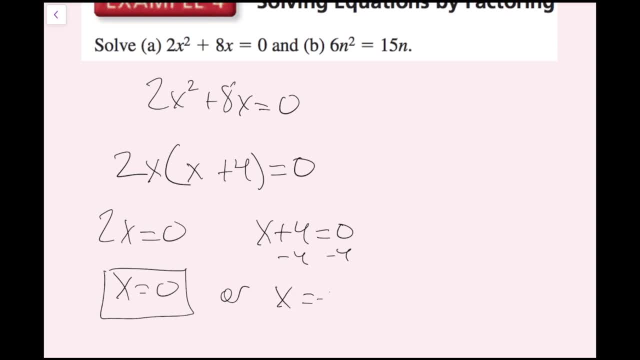 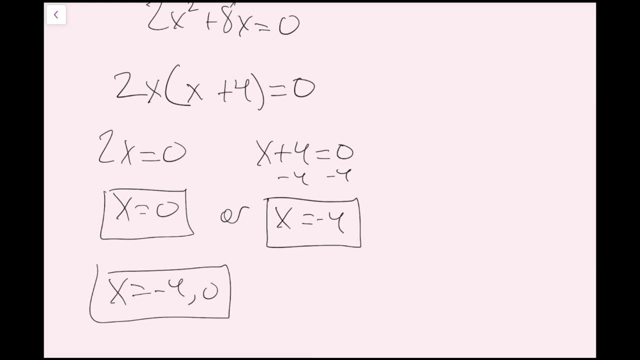 plus 4.. Well, if I subtract 4, I get x equals negative 4.. And once again you can write it like this: x equals negative 4, comma 0.. So now we're done with part A. For part B, I have 6n squared. 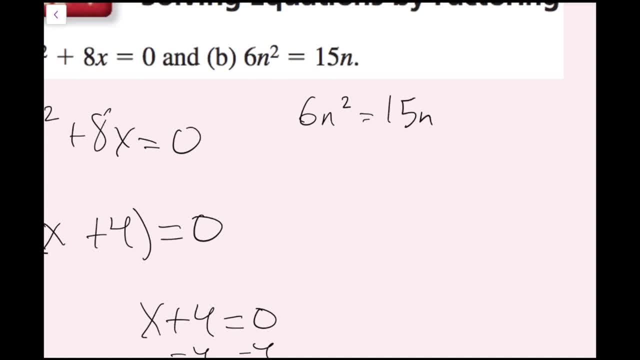 equals 15n. This one might be a little bit more complicated, but it's going to be a little bit trickier And I'm going to put some space in between that. And the reason is because we might want to say, oh, if I divide n, that would cancel out at least one of the n's. But we never want to. 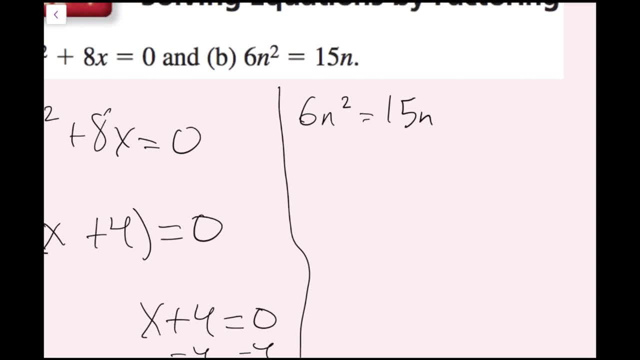 divide by a variable. We'd always rather factor, because we might miss some values if we end up dividing by a variable. So what I want to do is I want to get all my terms on one side and set them equal to 0, so I can hopefully use my 0 product property. So if I subtract 15n on both sides, 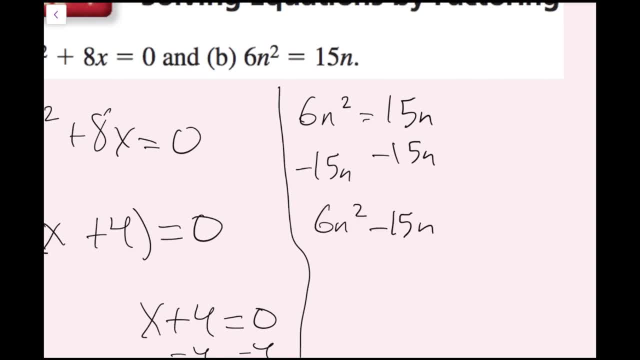 I get 6n squared minus 15n, And then this just cancels. Remember, canceling with addition and subtraction is 0.. So now I have 6n squared minus 15n equals 0.. And now I can find my greatest common factor to factor. 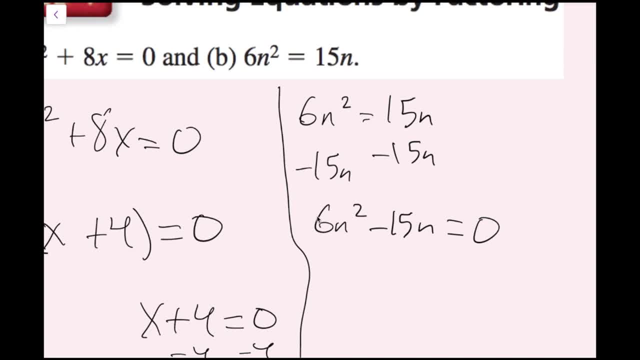 out, And then I can use my 0 product property. So I have a 6 and a 15.. I know I can factor out a 3 here, And then I have an n and an n squared, So I can factor out an n there And what's left is just. 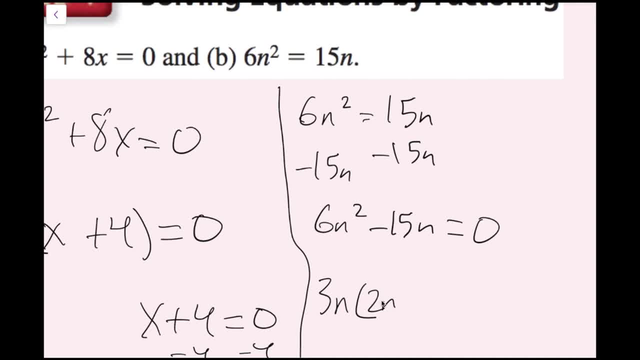 going to be 2n right here, because 3n times 2n is 6n squared, So I can factor out an n there And then this is going to be negative. So I do 3n times negative 5. I get negative 15n. 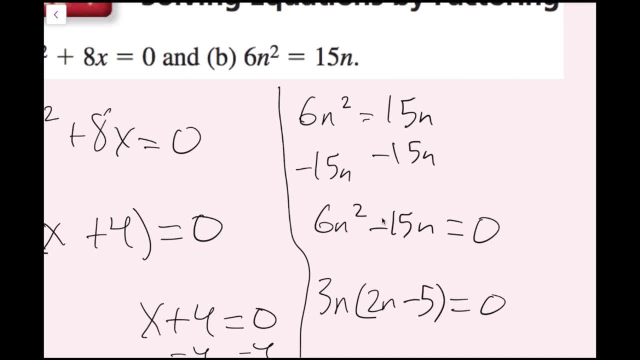 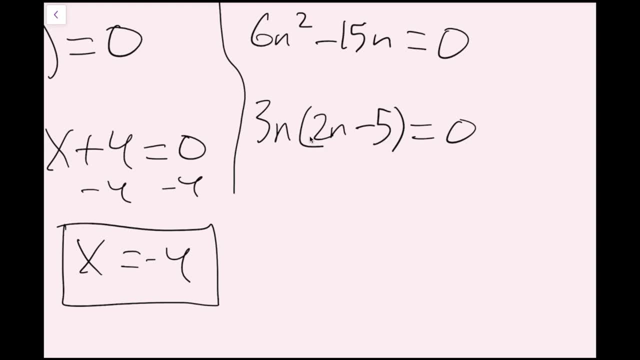 And if you're not sure, you can just distribute this out and see if it matches. Anyway, now I have two things that are being multiplied by each other that are equal to 0. I have 3n times the quantity 2n minus 5. So I can set these both equal to 0 by using my 0 product property. So 3n equals 0,. 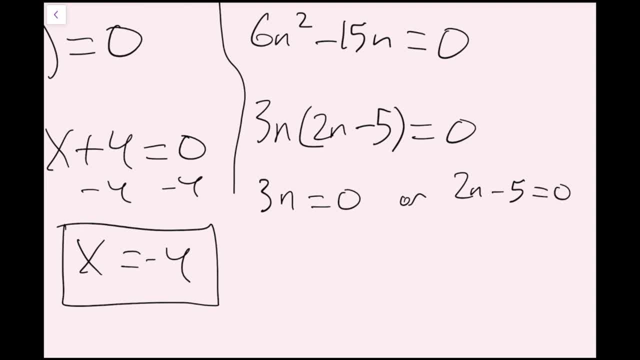 or 2n minus 5 equals 0. Now I can divide this equation by 3. Or you could have just been able to tell that n is going to equal 0 here. Or if I add 5 here and I get 2n equals 5, then I divide 2.. I get n equals 5. halves. 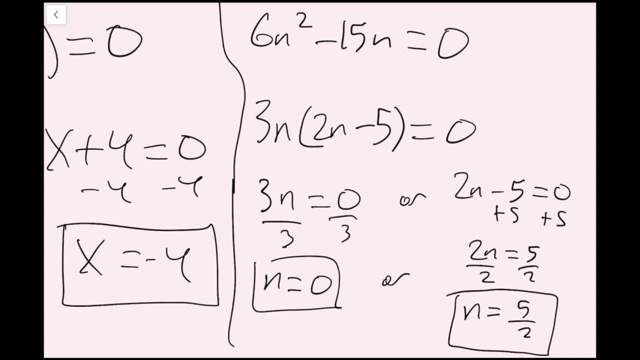 2.5, or 2 and 1 half. It doesn't matter which way you write it. Anyway, I could write my answer like this: n equals 0,, 2 and 1 half. I'm just going to do a mixed number here. You could have written: 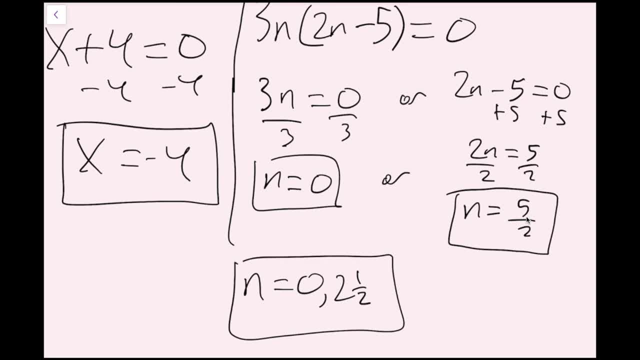 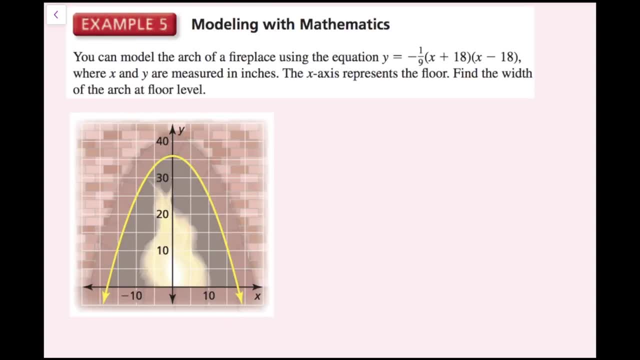 5 halves. That would have been fine too. Anyway, I have successfully solved this equation. I solved my equations by factoring first and then using the 0 product property, And now we're done with this one. For example, 5,. you can model the arch of a fireplace using the equation y equals. 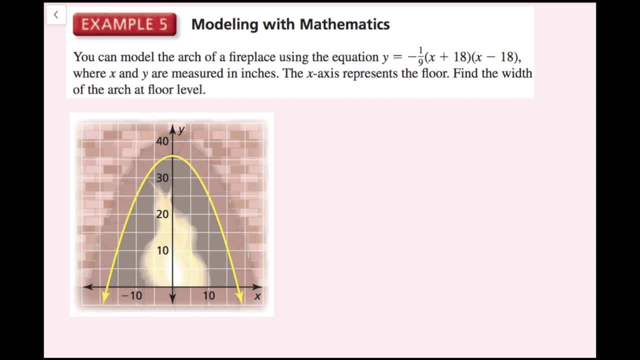 negative 1 ninth times quantity x plus 18 times quantity x minus 18,. where x and y are measured in inches, The x-axis represents the floor. Find the width of the arch at floor level. So what I'm trying to find is basically just how wide this fireplace is at the floor level. 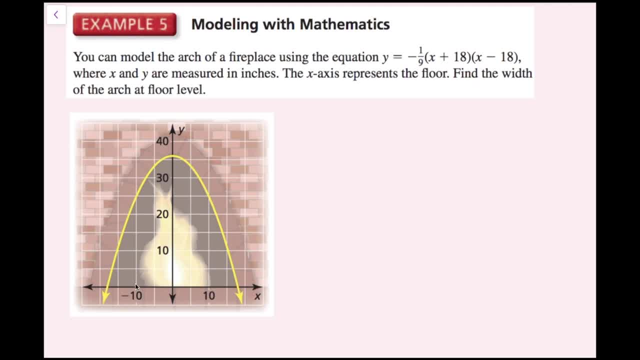 and we're treating the x-axis as floor level, okay, So I just basically need to find the distance between here and here. The problem is, I don't know what the exact value is between here and here by just looking at the graph, So I need to solve for that, okay, And what I'm going to do is actually 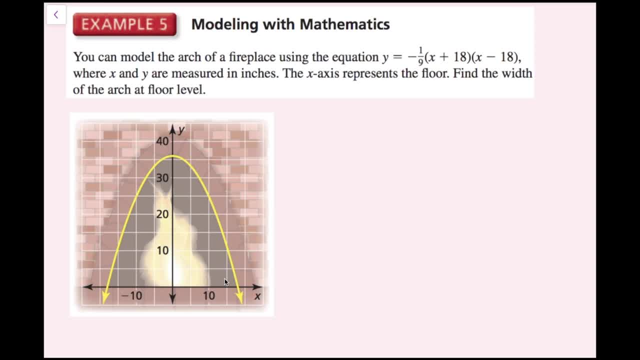 use the fact that I know that this floor is the x-axis, because I know that the x-axis right here is when y equals 0, okay, So to find what this x-value is and this x-value is, I can just set 0.. So I'm going to rewrite this equation, but y is going to be equal to 0,, once again because of the. 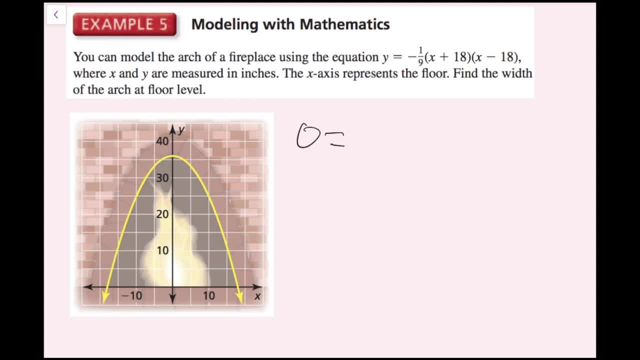 x-axis is when y is 0. So I'm going to rewrite: 0 equals negative 1 ninth times x plus 18 times x minus 18.. And now I'm going to solve this. Well, I have a number that's being multiplied here. 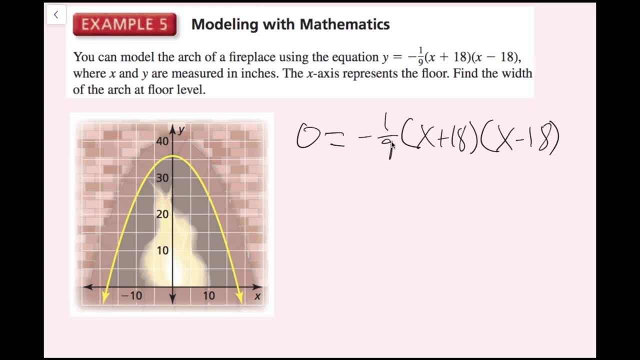 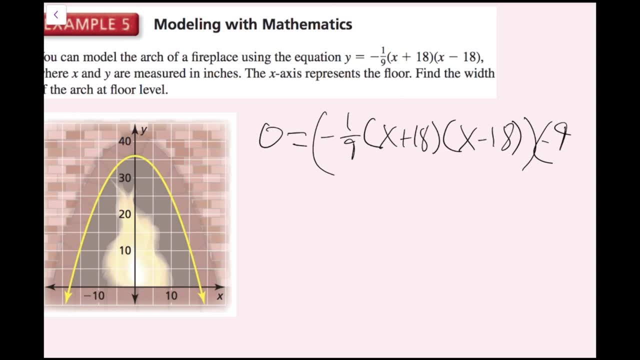 but if you see, I can just get rid of this, because if I multiply both sides of this equation by the reciprocal of this, which is going to be negative 9,, to cancel that out, negative 9, on both sides. Well, negative 9 times 0 just stays 0. And then this negative 9 and this negative 1. 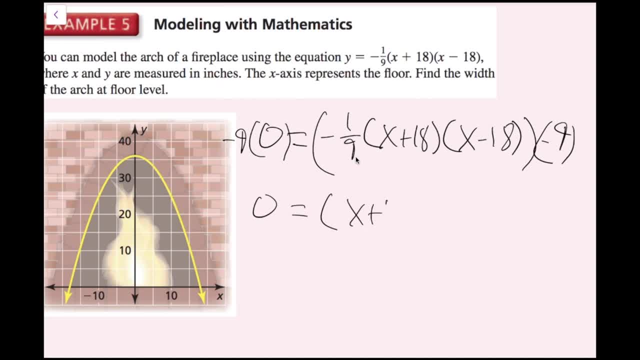 ninth: just cancel. So all I have left now is x plus 18 times x minus 18 in parentheses. okay, And now I can use my 0 product property. So I'm going to set x plus 18 equal to 0.. 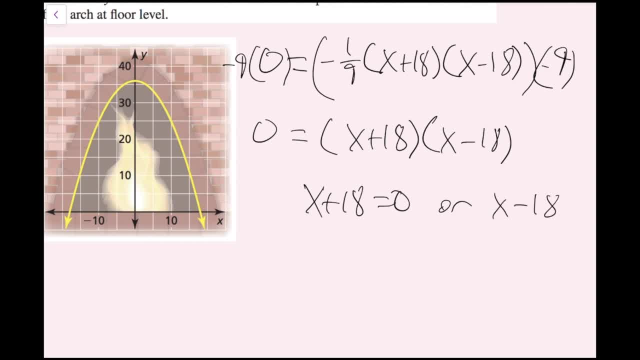 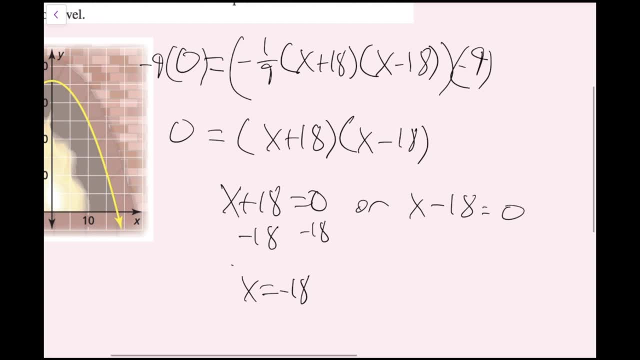 And I'm going to set x minus 18 equal to 0. And if I subtract 18 here I get x equals negative 18. So that's one of my x values. And then if I have adding 18 here, I should say I get x equals positive 18.. So I know my two x values.